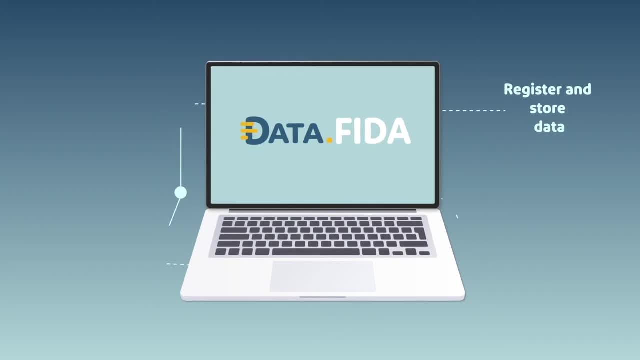 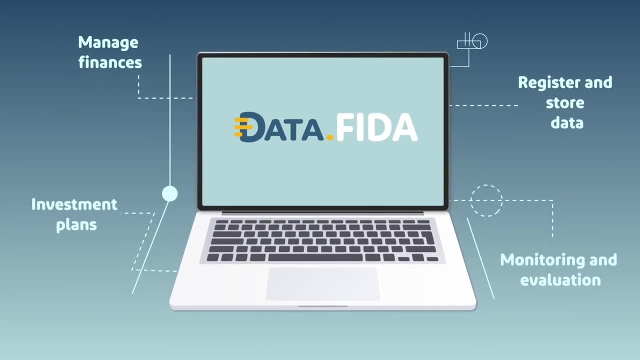 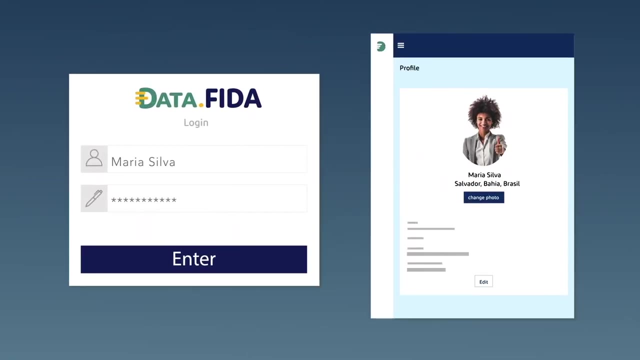 In this intuitive platform, you can register and store data, manage finance and investment plans, perform monitoring and evaluation, all in an agile and transparent way. Start customizing your profile. You can add your photo and personal information. The DataFeeder has three distinct interfaces to meet the specificities of its users. 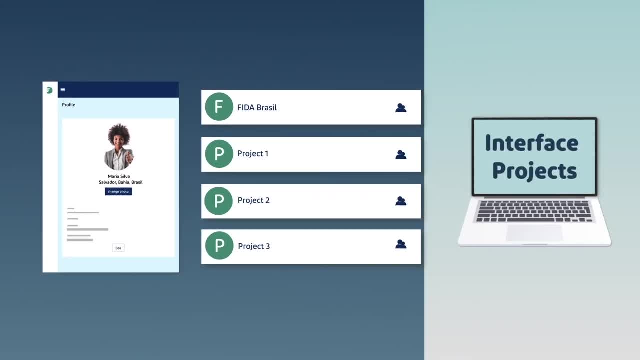 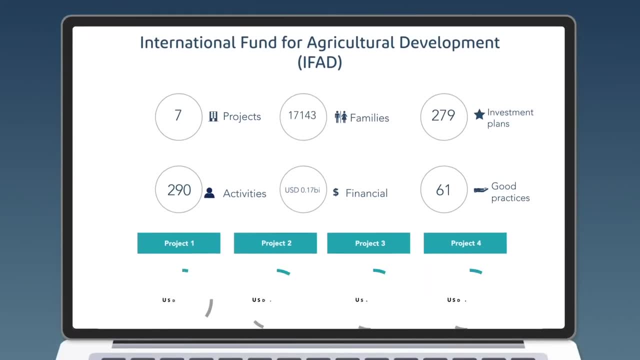 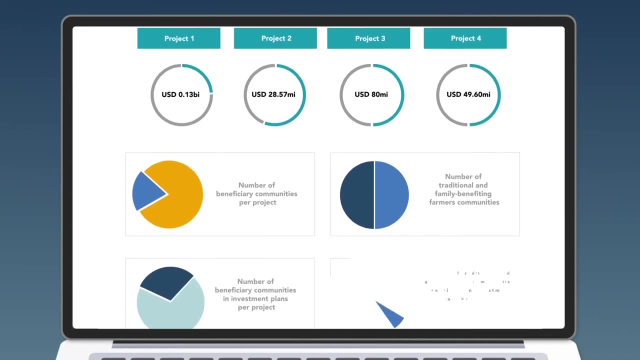 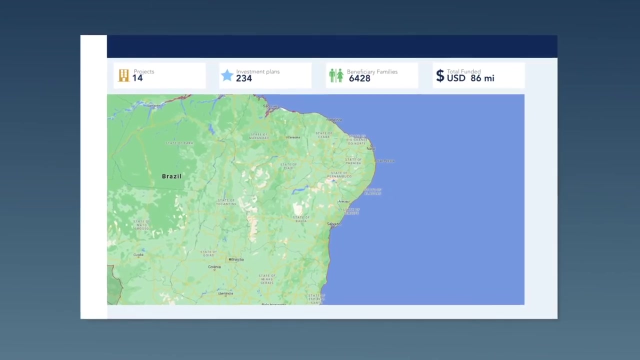 The public interface, the IFAD interface and the project interface. The public interface is intended for all those people who are interested in agricultural development. It offers the results of each project supported by IFAD in Brazil, as well as information on good practices. The IFAD interface allows staff and consultants. 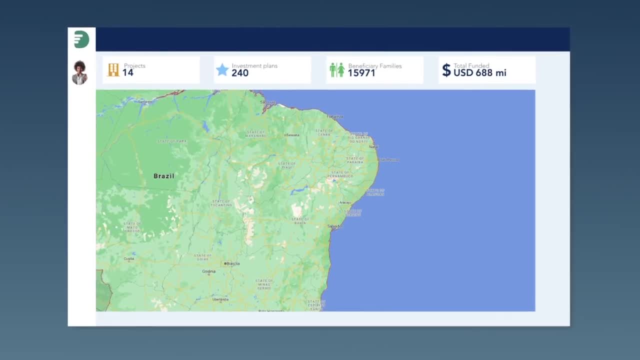 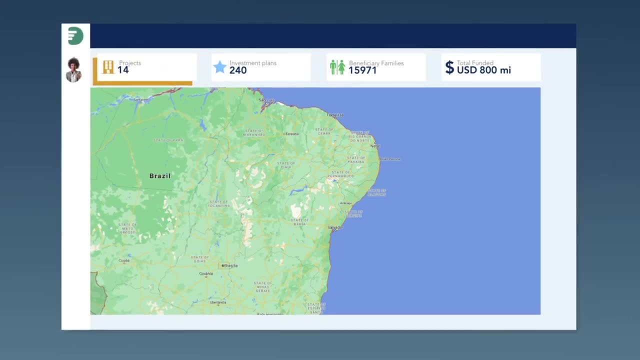 from the fund to follow the development of each project in all stages. Here you can see the number of projects developed in Brazil, the number of families benefited, the investment plans and the total already financed by IFAD. Maps, charts and tables make the visualization easier. 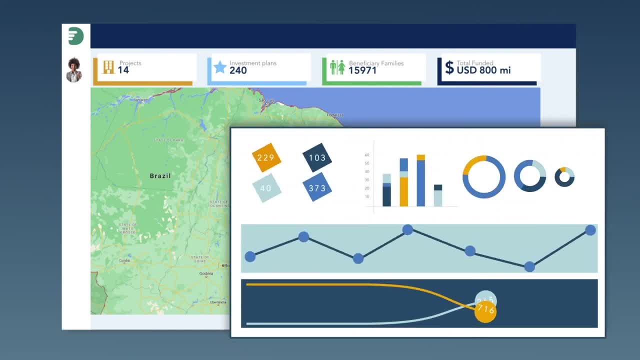 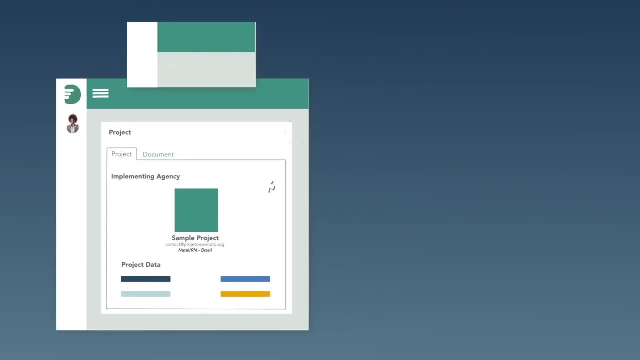 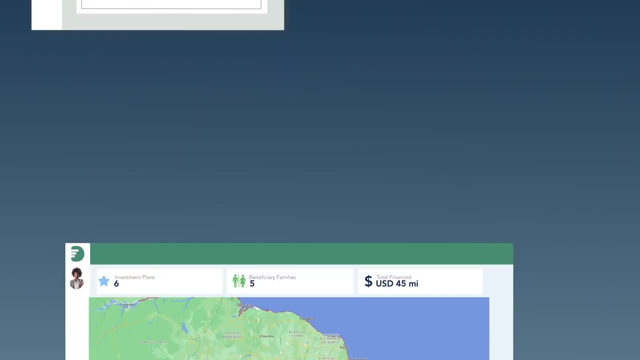 and the navigation light and enjoyable. The project interface was specially designed for those who manage the projects with tools that facilitate the daily routine and enhance the work. Navigation begins in the dashboard, where you can place the beneficiary entities, communities and people on the map. 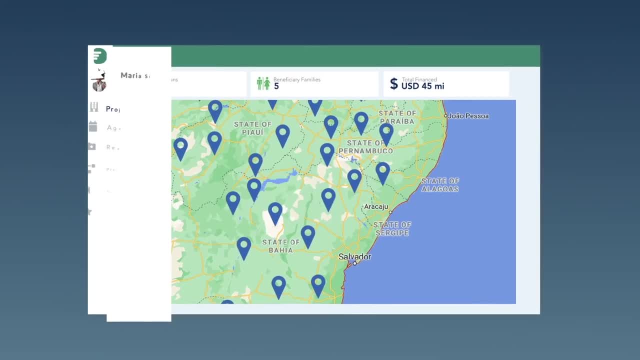 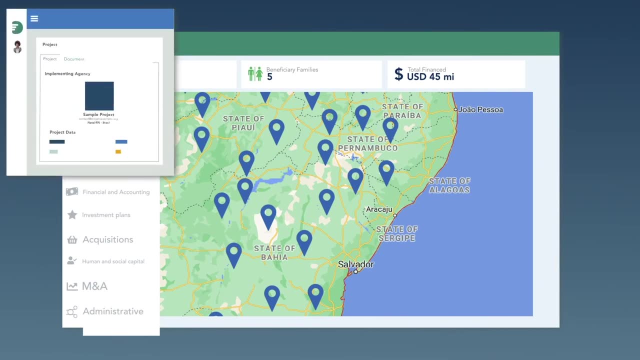 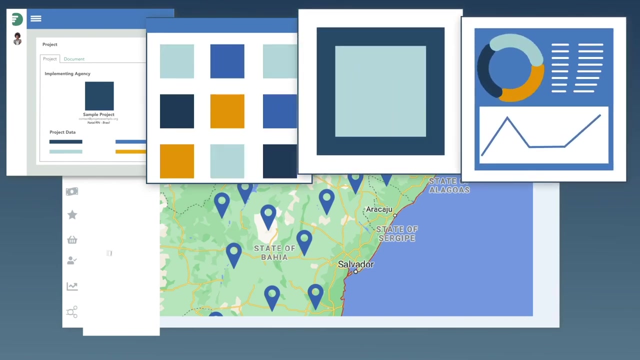 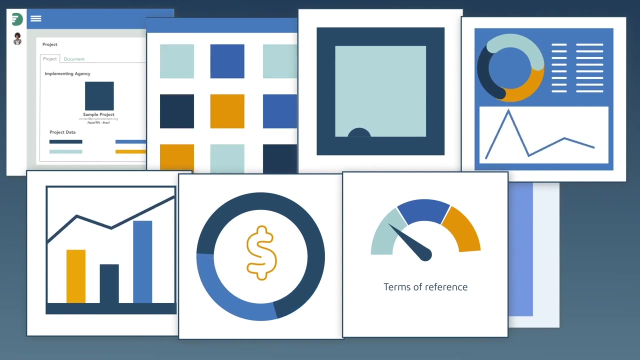 through geolocation. by clicking on the modules that appear in the side menu, the manager can perform different tasks: check project data and documents, schedule and view events, register people and user groups. manage the project. manage the finances, track investment plans. manage terms of reference bids and contracts, register activities and events held. monitor and evaluate key project. 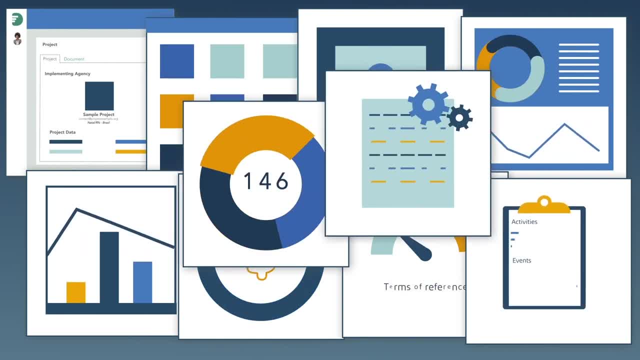 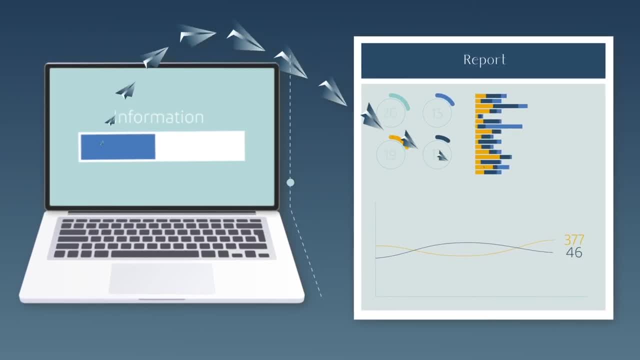 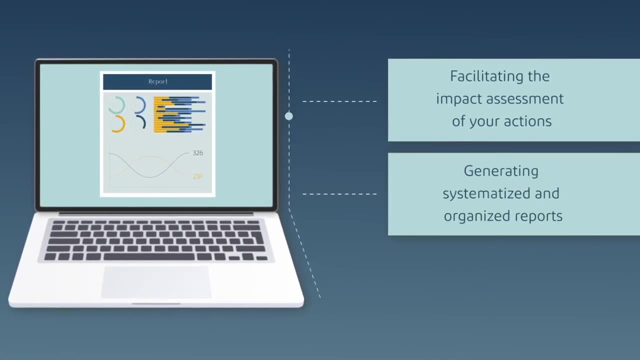 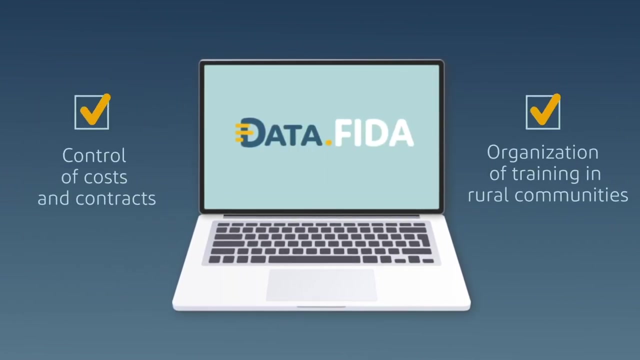 indicators, document and track actions related to the use of the system, updating the information during the execution of your project. the platform groups, all data facilitating the impact assessment of your actions and generating systemized and organized reports, from cost control and contracts to the organization of training in rural. 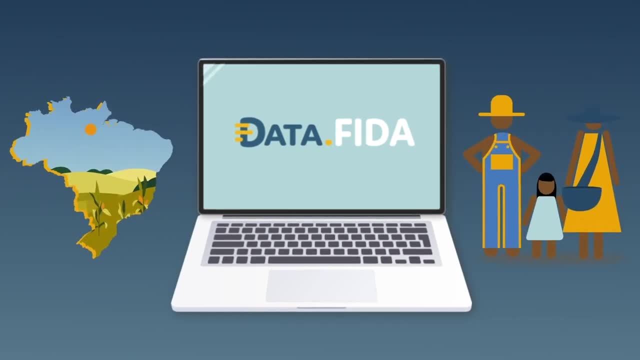 communities data feeder has come to definitely change project management.